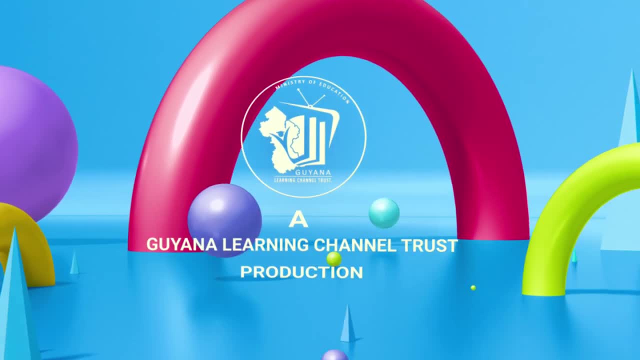 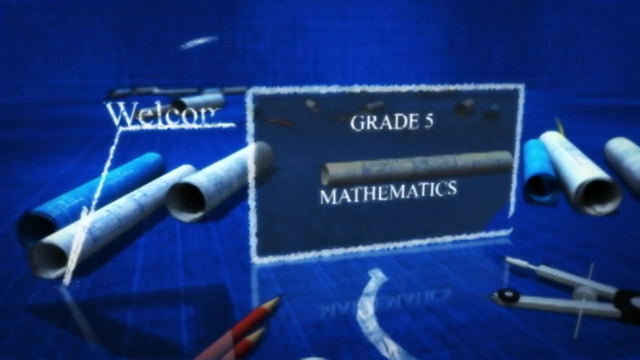 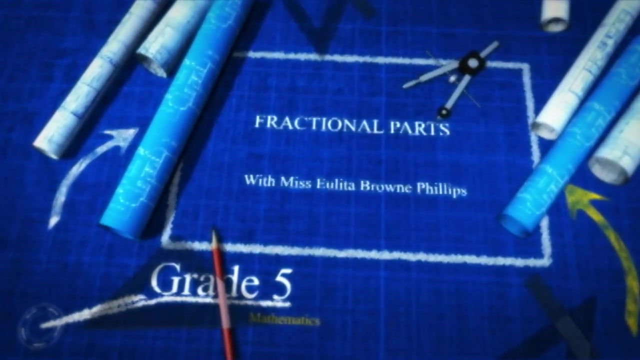 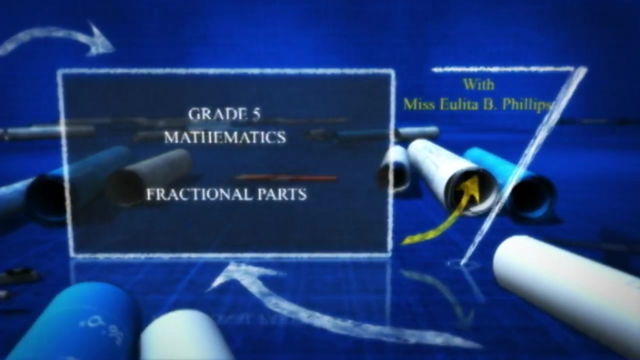 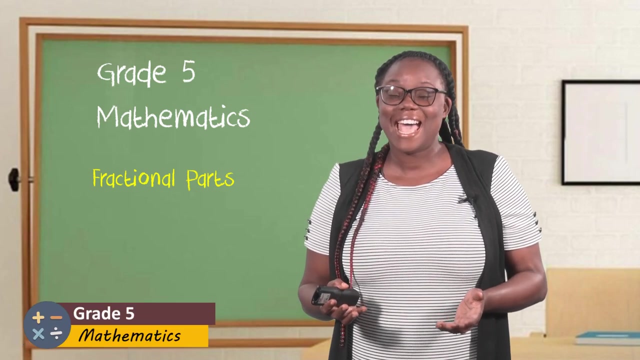 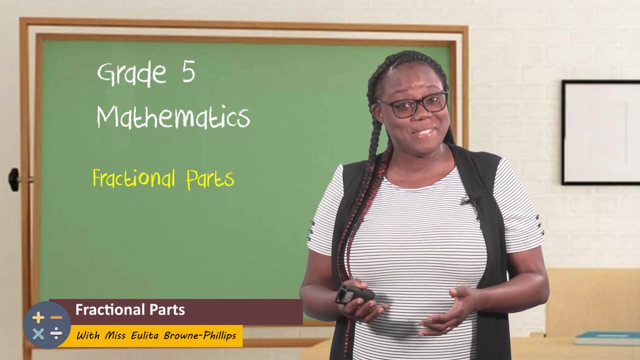 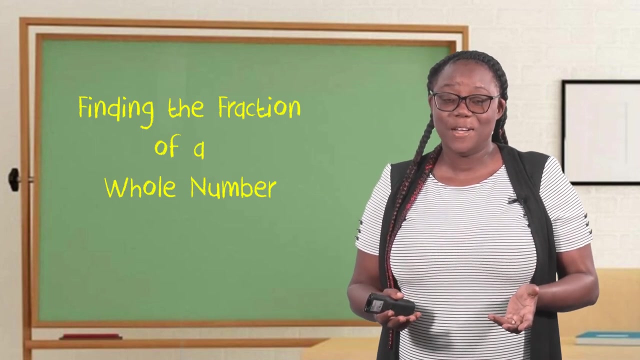 Hello, boys and girls of grade 5.. Welcome to our mathematics class. I am Ms Yulita Brown-Phillips. How have you been, boys and girls? I hope that you have been staying safe and healthy. Our topic for today would be finding the fraction of a whole number. 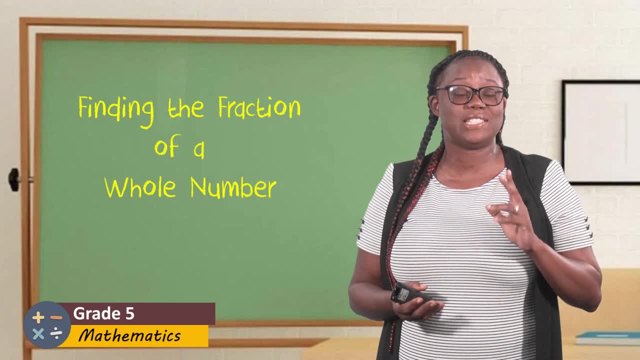 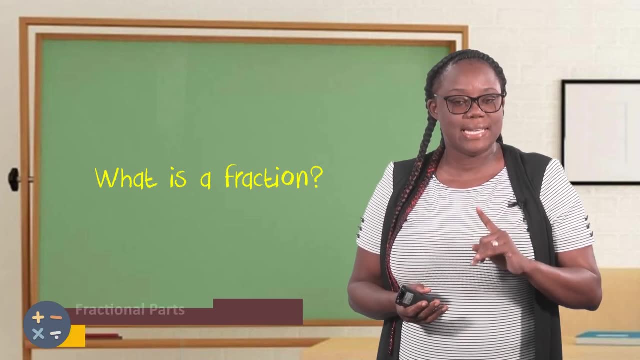 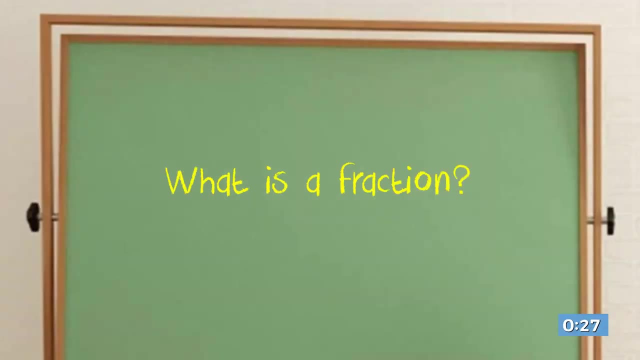 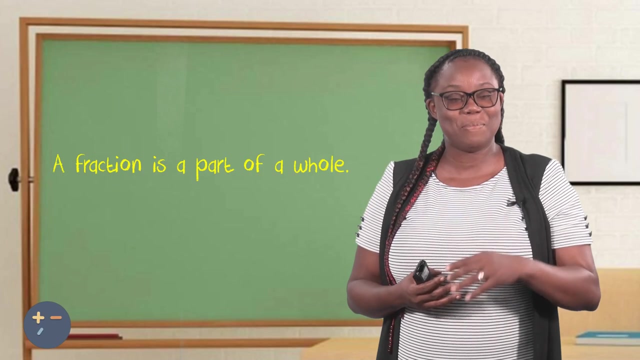 But, boys and girls, you know that it's customary, before we get into our topic for the day, that we do a bit of recap. Do you remember what is a fraction? I'll give you two seconds to think about it. Yes, boys and girls, Did you say? a fraction is a part of a whole. 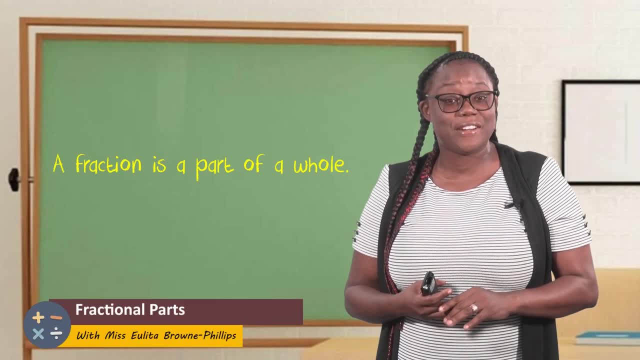 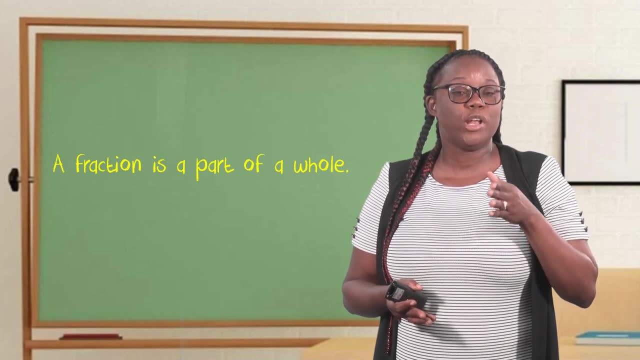 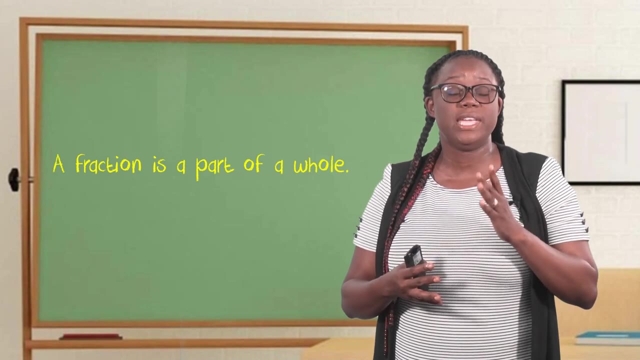 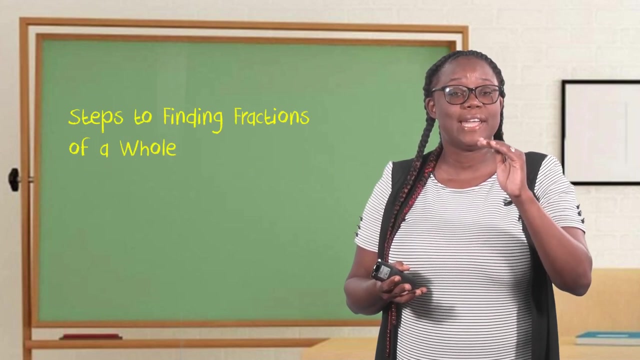 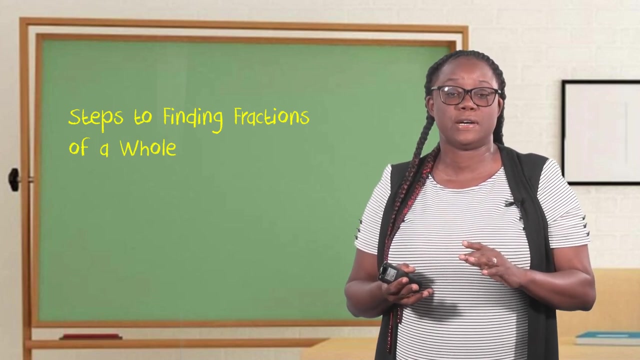 Well, you are absolutely correct. A fraction is a part of a whole. Now remember, we always say that in mathematics we have to do everything step by step So that we can arrive at the correct answer. So today we are going to look at the steps to finding fractions of whole numbers before actually working it out. 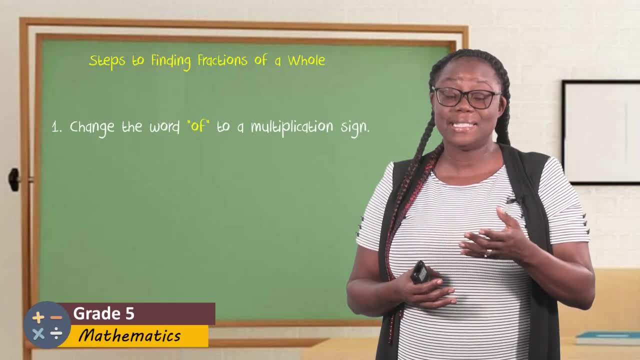 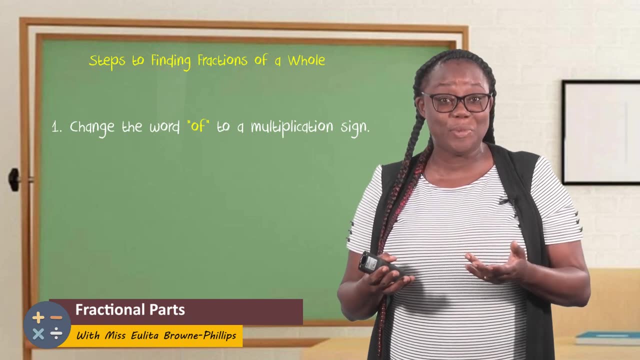 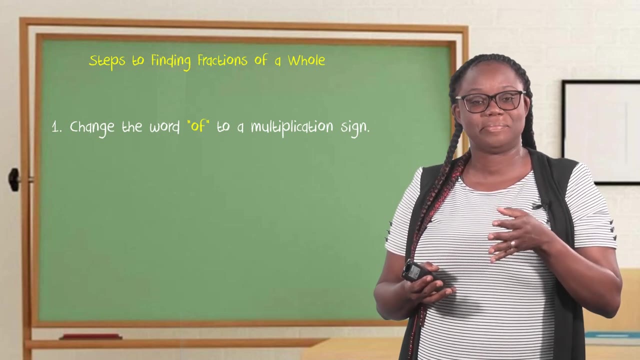 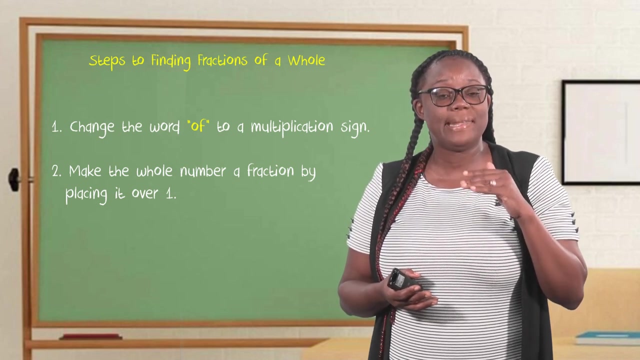 Step 1. In mathematics, the word of means multiply. So the first thing you do, boys and girls, is to choose. So you change the word of to a multiplication sign. Our next step: We make the whole number a fraction by placing it over 1.. 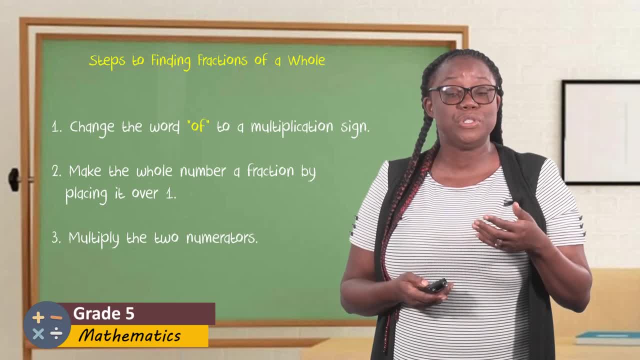 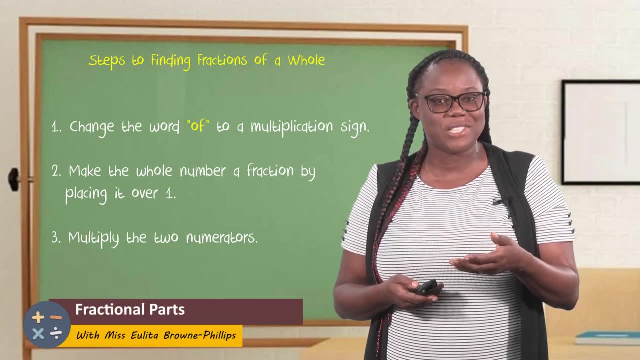 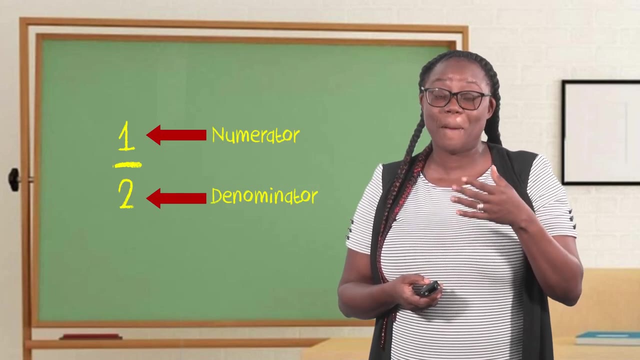 Then we multiply the two numerators, Boys and girls. I'm a bit curious. Do you remember where the numerator of the fraction is located? Yes, it is the number at the top and the number at the bottom. it is the denominator. 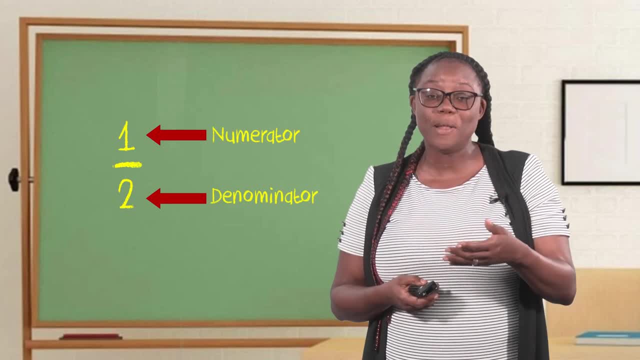 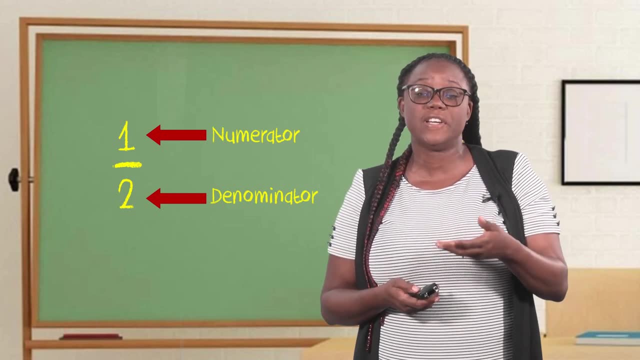 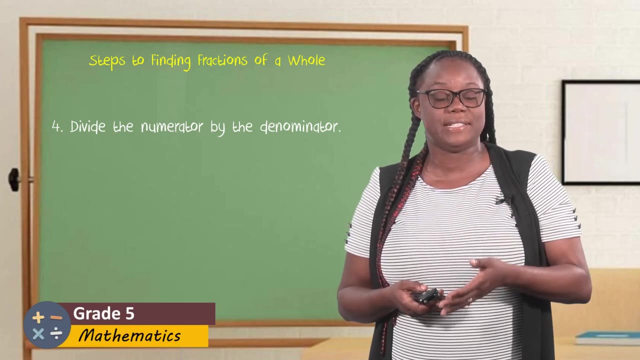 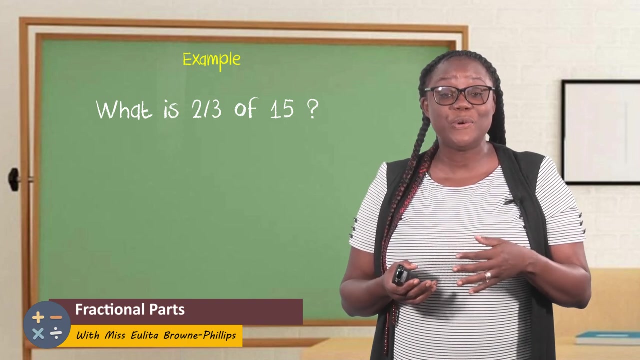 That number tells us how many equal parts the shape is divided into, or how many equal parts the fraction has. The final step is to divide the numerator by the denominator. So let's look at this example question Quickly: What is 2 thirds of 15?? 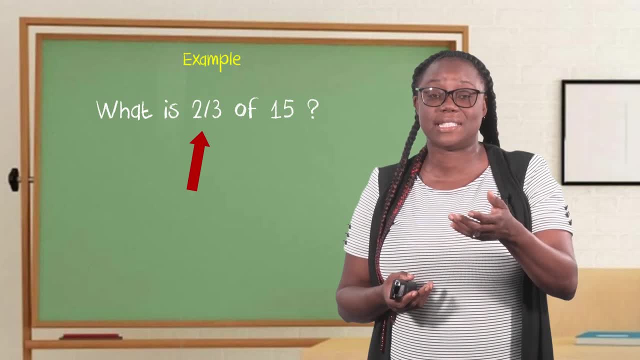 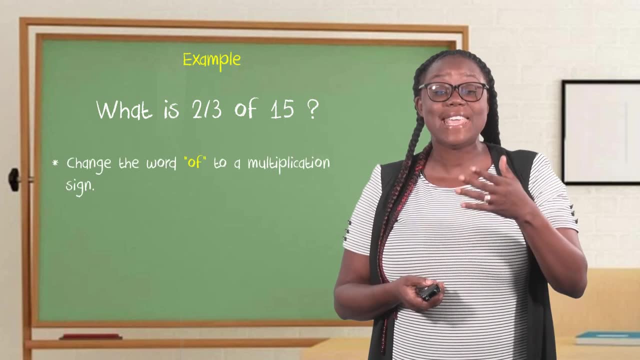 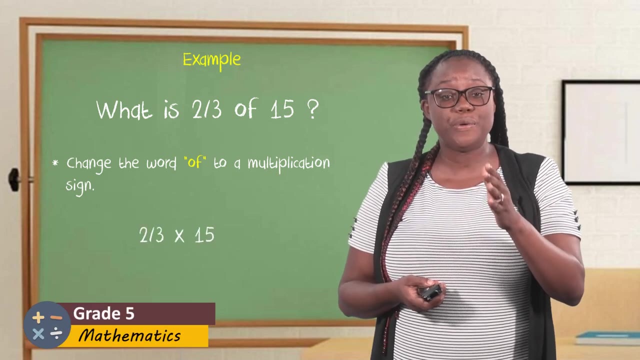 We know that the fraction there is 2 thirds. We know that the whole number is 15.. What did our first step say? Yes, we changed the word of to multiply. So it's 2 thirds multiplied by 15.. So it's 2 thirds multiplied by 15.. 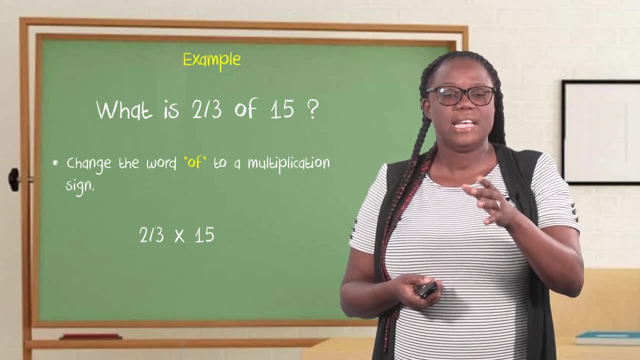 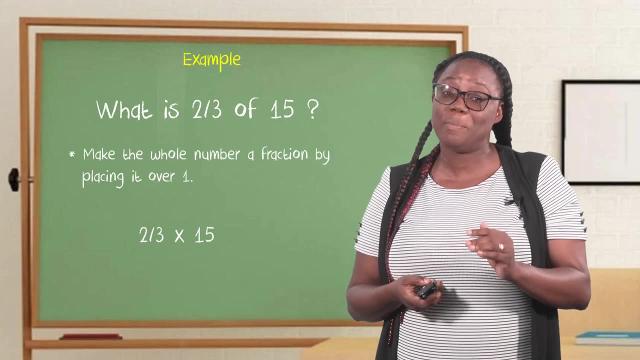 So it's 2 thirds multiplied by 15.. The next step said something. The next step said something. Do you remember what it said? Yes, we make the whole number a fraction by placing it over 1.. Yes, we make the whole number a fraction by placing it over 1.. 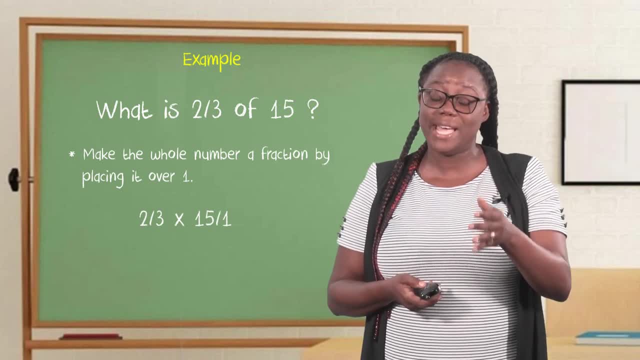 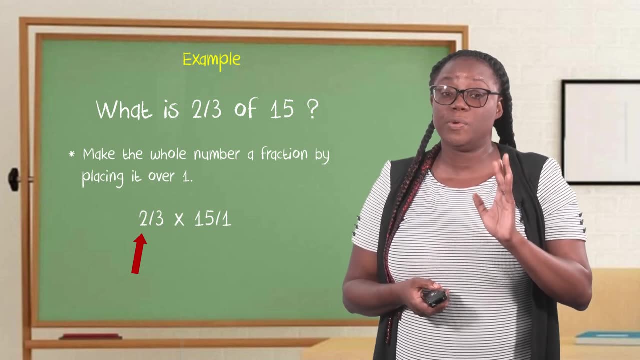 Now we can begin to work. Now we can begin to work. We multiply our numerators. We multiply our numerators, So our numerators are 2 and 15.. So our numerators are 2 and 15.. 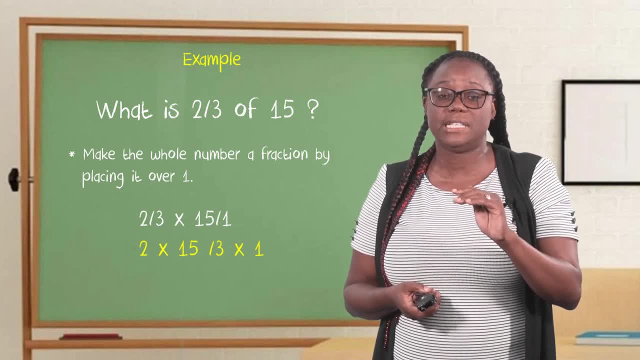 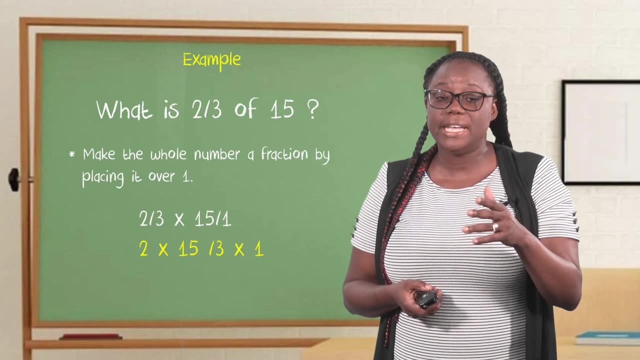 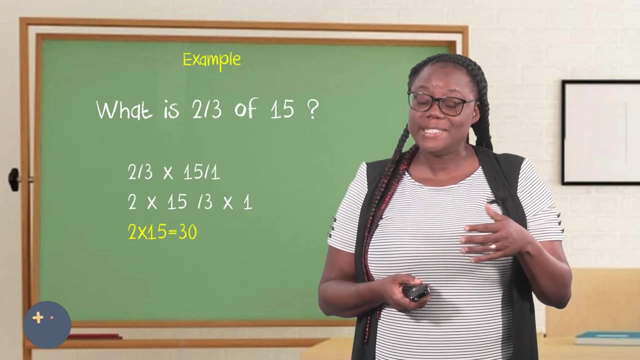 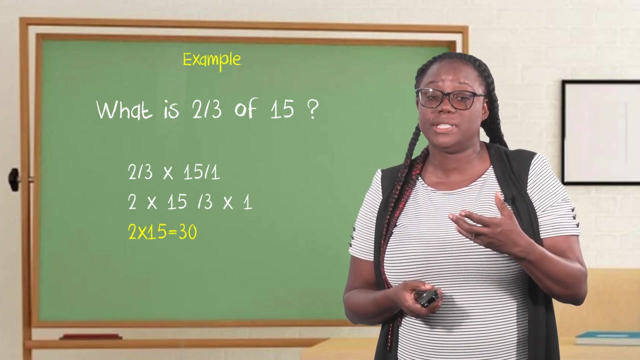 So we will have 2 multiplied by 15, by 15 then we multiply our denominators over 3 times 1, so let's continue to work. 2 times 15 will give us 30, so 30 becomes the numerator. 3 times 1 will give us 3. 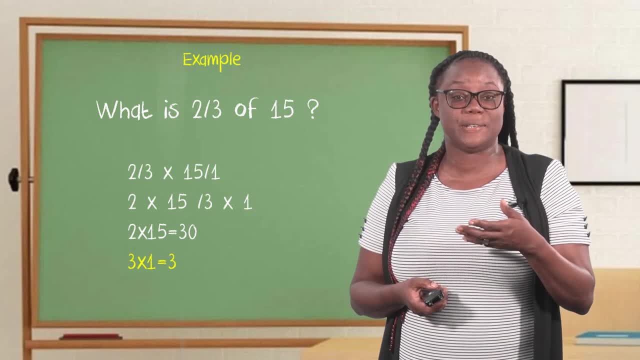 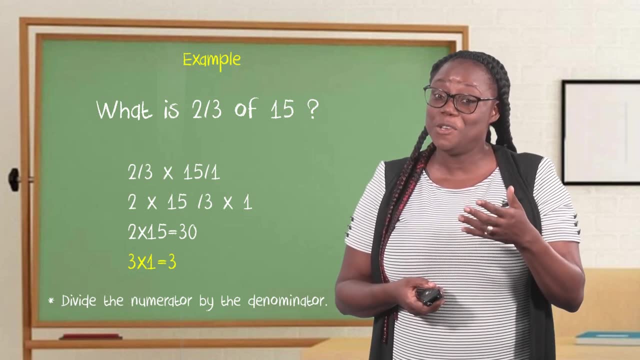 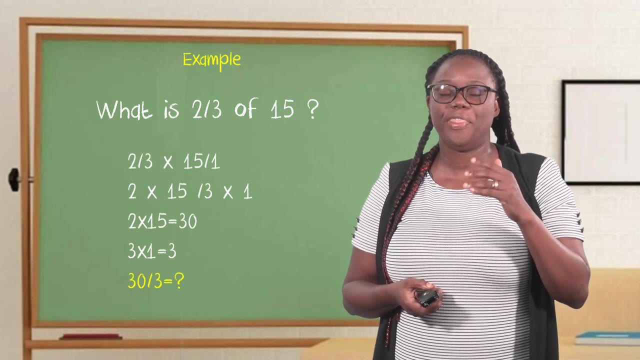 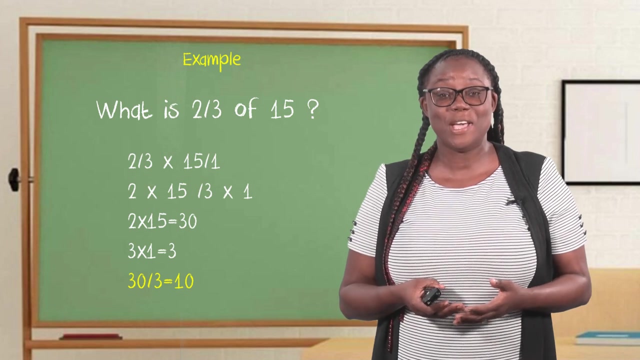 so 3 becomes the denominator. now it's time for the final step, which said: divide the numerator by the denominator. so it's 30 divided by 3. how many groups of 3 can you get from 30? yes, boys and girls, we can get 10 groups of 3 from 30. so there, 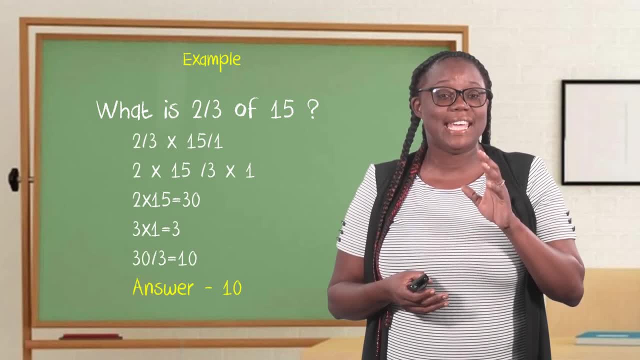 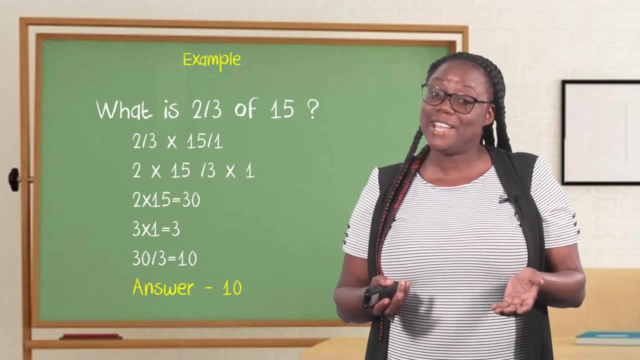 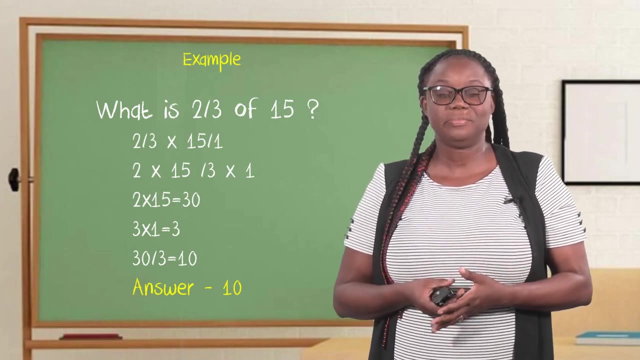 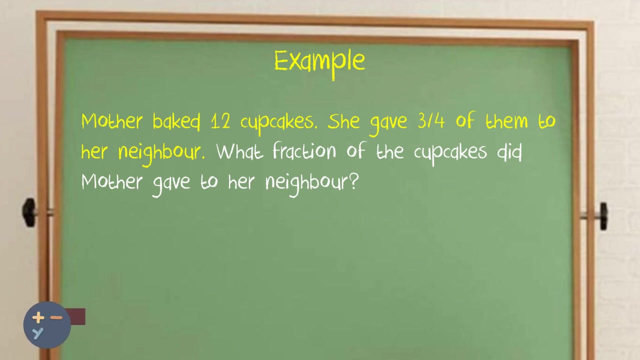 four. two-thirds of fifteen is ten. Pretty easy, don't you agree? So we're gonna do another example, but this time this example- you will have a worded problem. Mother baked twelve cupcakes. Boys and girls, do you like cupcakes? Yummy, I love cupcakes. She gave three-fourths of them. 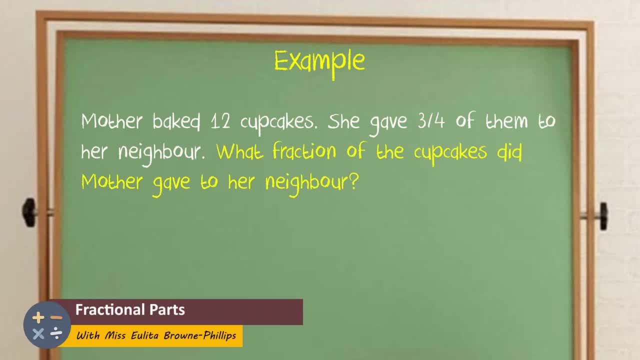 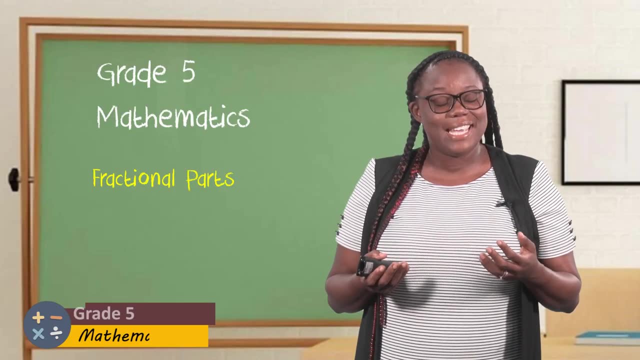 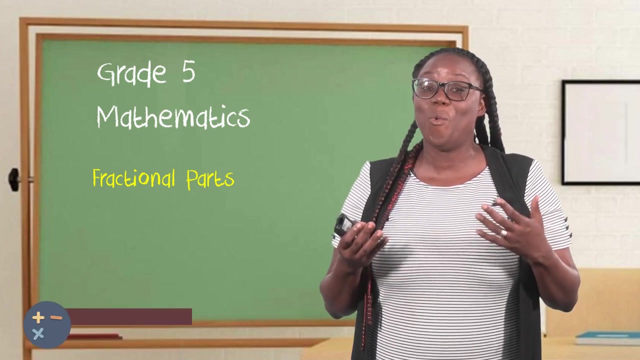 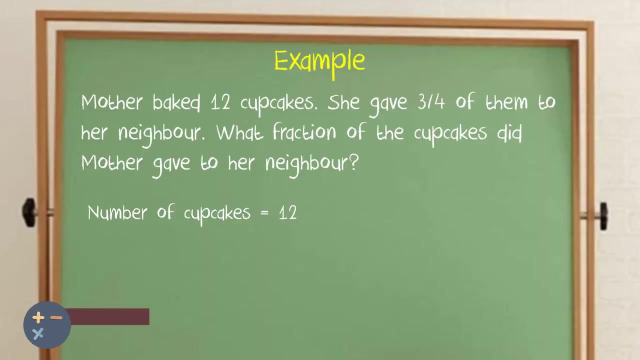 to her neighbor. What fraction of cupcakes did mother give to her neighbor? Boys and girls. in mathematics, it's advised that you must read your problems carefully so that you will understand what is required of you. So, first off, how many cupcakes did mother bake? Number of cupcakes. 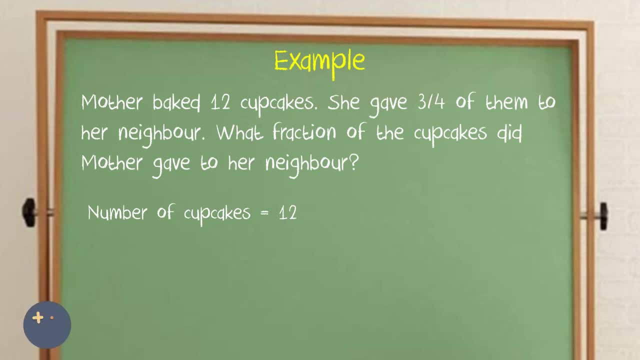 equal twelve. What fraction of the cupcakes did mother share? She shared three-fourths of the cupcakes. So therefore, the number of cupcakes shared is three-fourths of twelve. Let's go to the solution: Three-fourths of twelve. Do you remember what we said about the word of in mathematics? 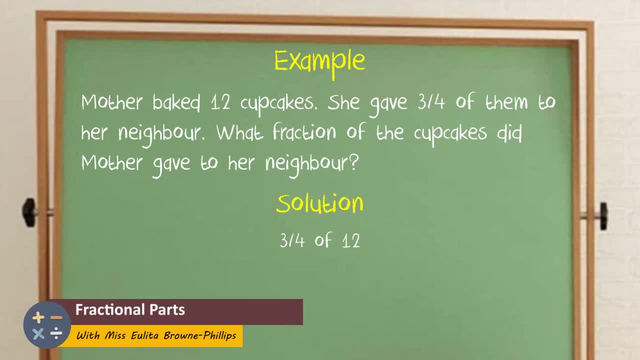 Yes, We changed the of to a multiplication sign, So we will now have three-fourths times twelve. Next step: We make the whole number a fraction by placing it over one. Three-fourths times twelve over one. Now we can work. So we will multiply the numerators. The numerators are: 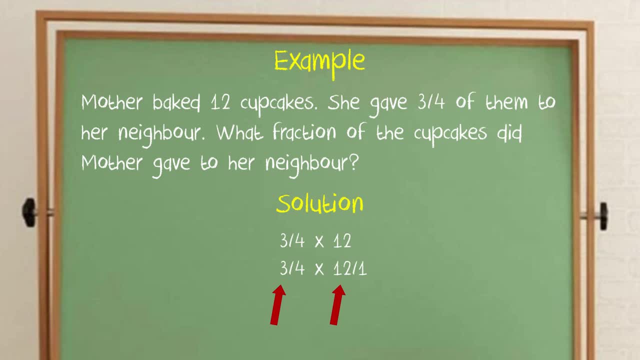 three and twelve respectively. Then you have the denominators four and one respectively. Three times twelve will give us thirty-six. Four times one will give us four. So our denominator becomes four and our numerator becomes thirty-six, 36.. Boys and girls, how many groups of four can we get from the number 36?? 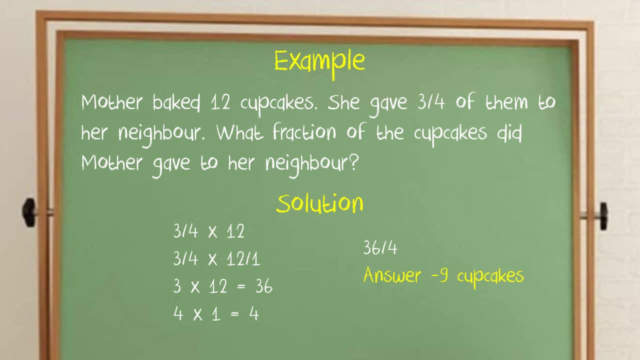 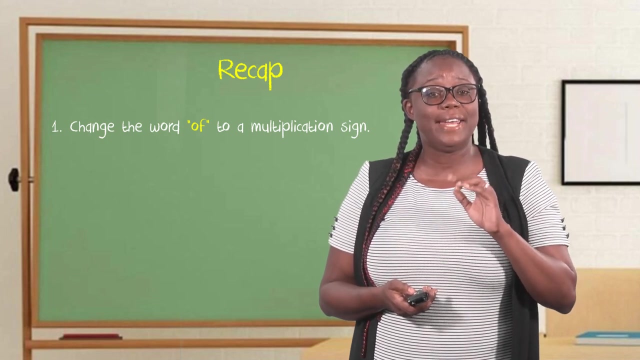 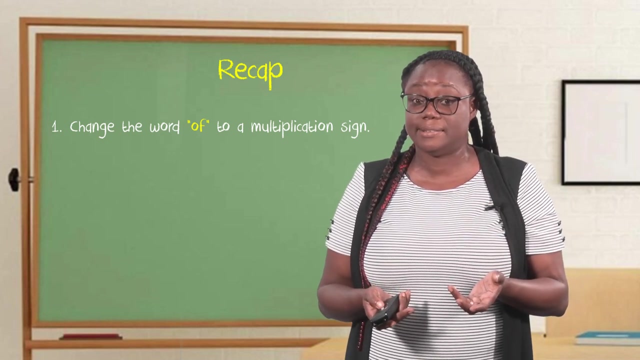 Did you say nine? You are absolutely correct. So mother gave nine cupcakes to her neighbor. So three-fourths of 12 is nine. Now let's recap. Remember: when finding fractions of quantities, the word of is changed to a multiplication sign. You make the whole number. 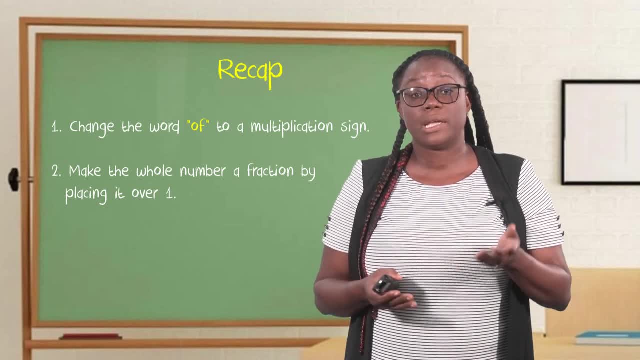 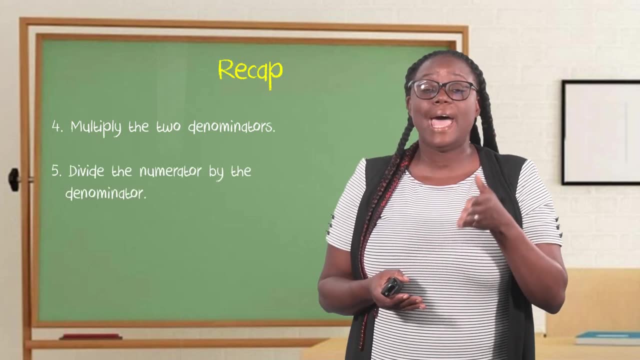 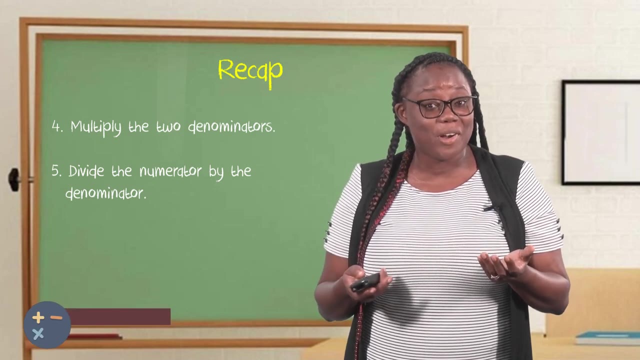 fraction by putting it upon one. We multiply the two numerators, Then multiply the two denominators, And then we divide the numerator by the denominator And we have our answer. Pretty simple, right, boys and girls? Yes, I know that you would have. 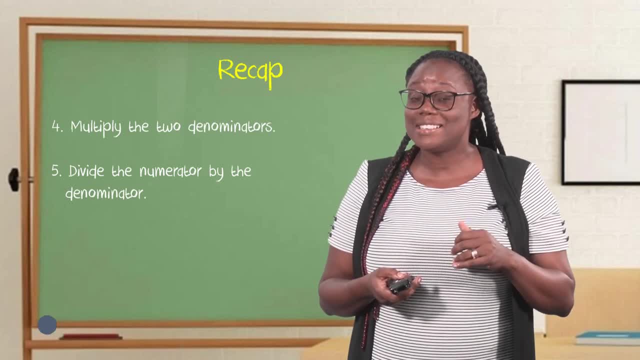 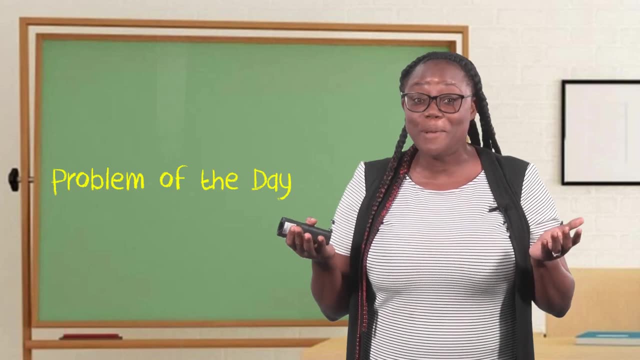 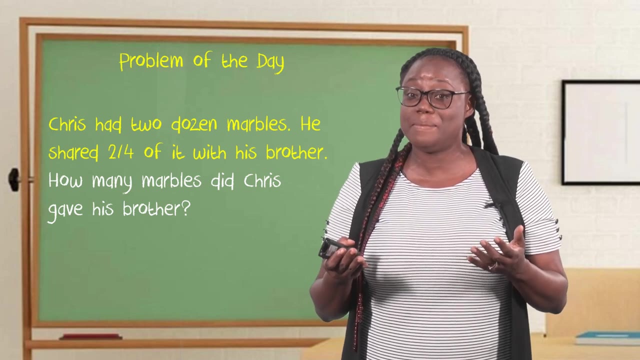 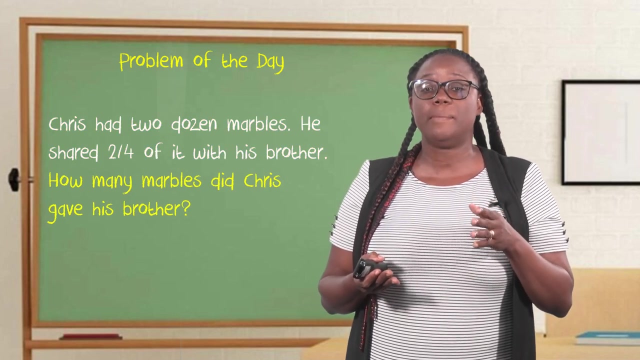 learned quite a lot today. But, boys and girls, guess what it's time for? You know we can never conclude our lesson without the problem of the day. So let's look at our problem of the day. Chris had two Dozen marbles. He shared two-fourths of it with his brother. How many marbles did Chris give to? 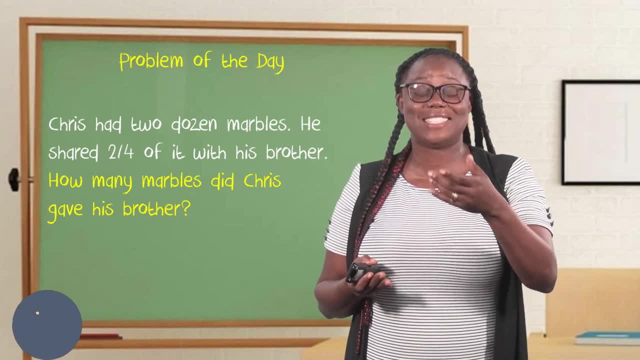 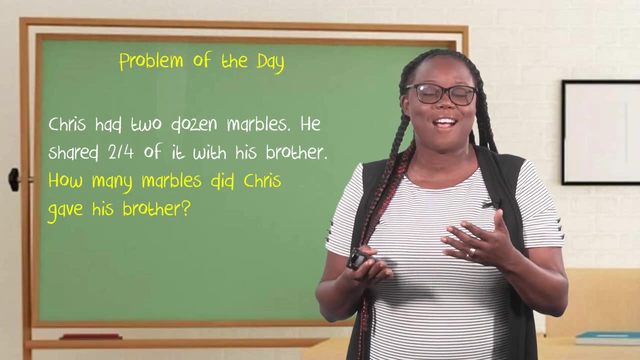 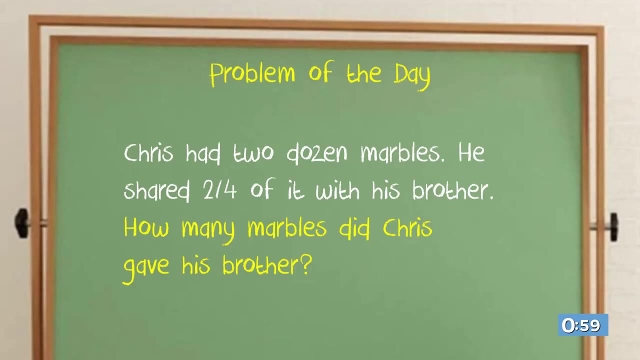 his brother, Boys and girls. it is now your turn to solve this problem. I am confident that you will be able to solve it, because you are excellent problem solvers, So take a minute and solve this problem, All right, And you canmänd me take two-fourths. 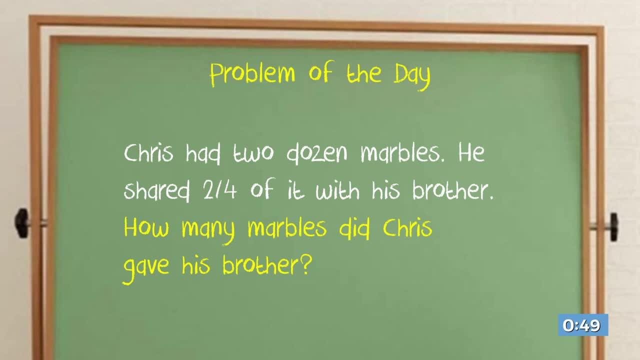 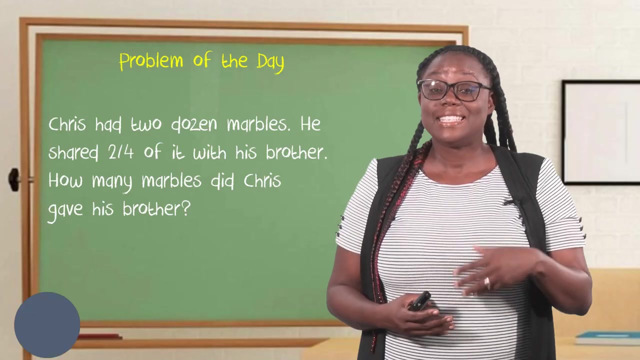 Therefore, I give you 3. Yep, Alright, So I take two-fourths of it. I take 3. 1. 1., 1., 1., 1. 1.. So, boys and girls, you should be finished by now. 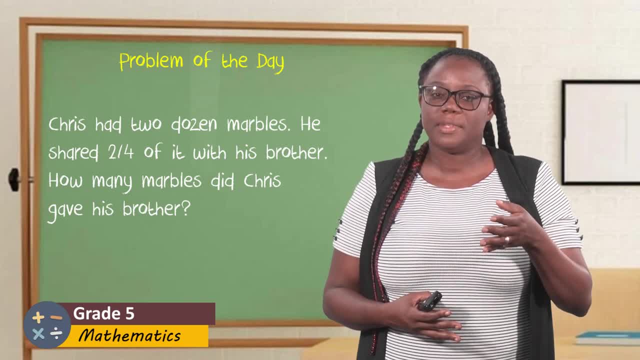 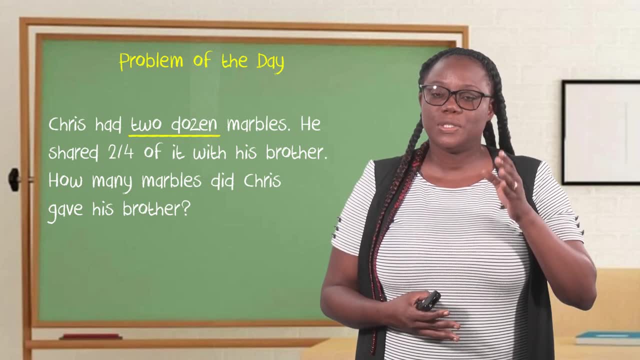 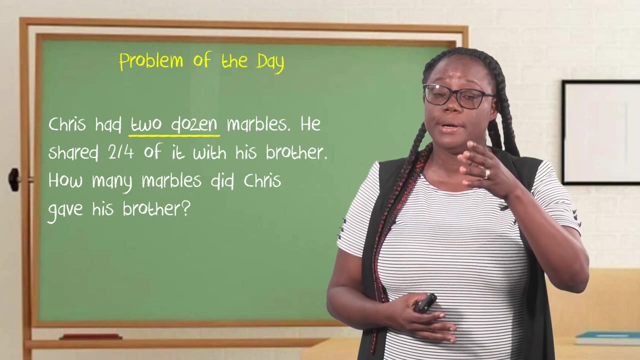 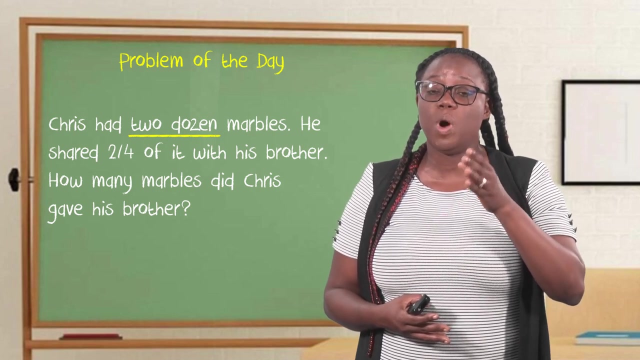 But before we work this problem we have to figure out how many marbles exactly Chris had. So we know that he had two dozen marbles, but we would like to have a whole number to represent that. So we now have to figure out how many things make one dozen. 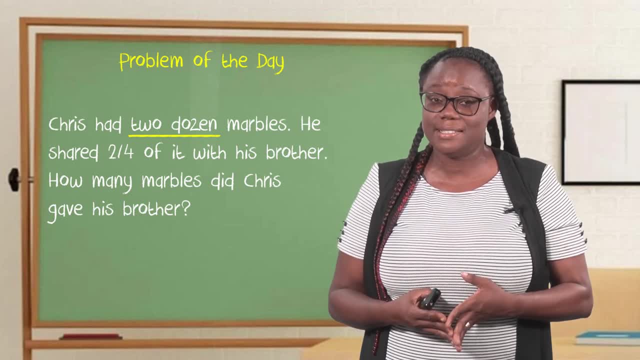 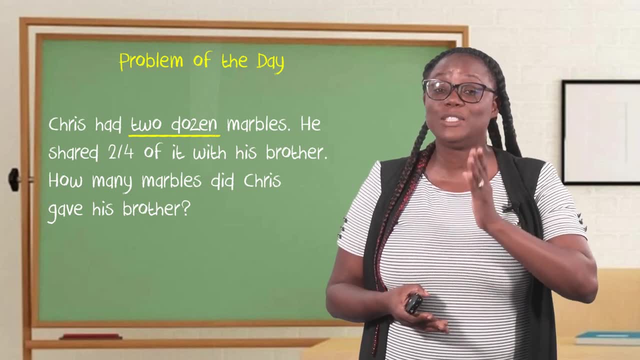 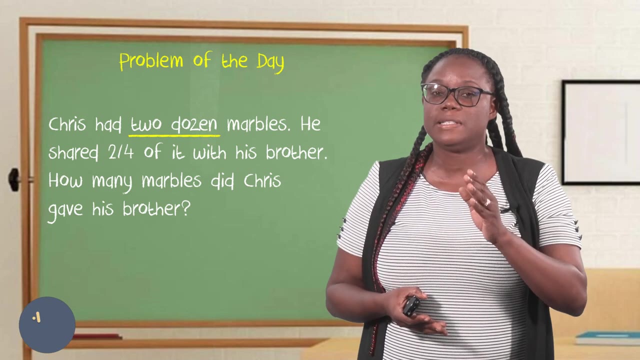 Boys and girls, do you know how many things make one dozen? Yes, twelve things make one dozen. So if Chris had two dozen marbles, to find out how many marbles Chris had, you would have to multiply twelve by two, which would give you twenty-four. 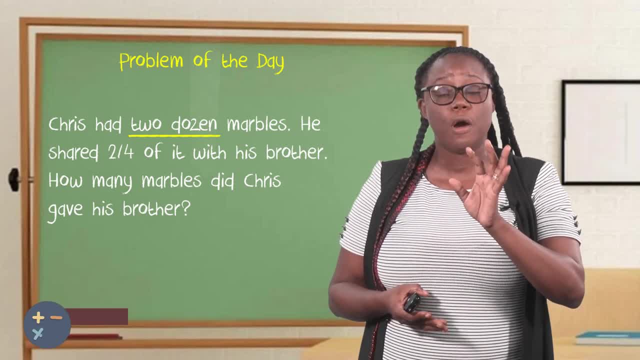 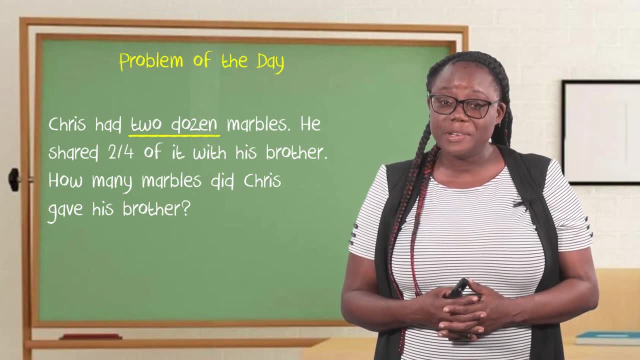 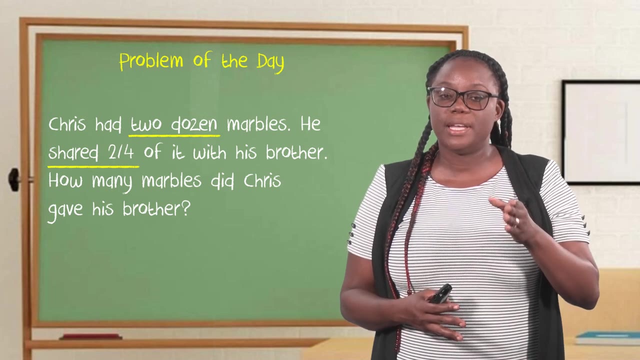 So the whole number in this problem would be twenty-four. Boys and girls. do you have twenty-four? Good job. What fraction of the marbles did Chris share Two-fourths? So our problem now is to find two-fourths of twenty-four. 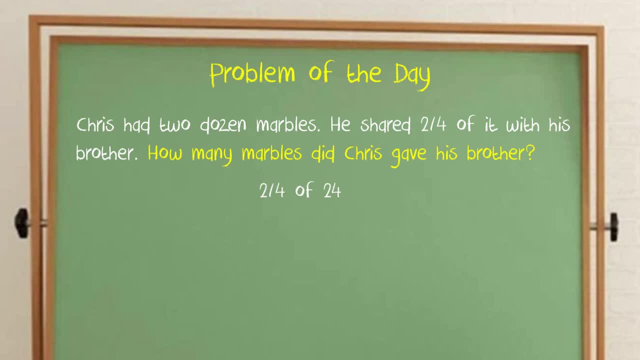 First step: we change the of to a multiplication sign, So it becomes two-fourths multiplied by twenty-four. Next step: we change the whole number to a fraction by placing it over the other side, So it's going to now be two-fourths times twenty-four over one.